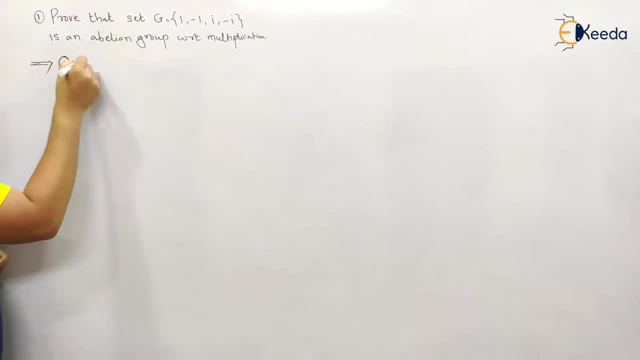 this set here. that is, of course, multiplication. So what is the first property that we need to prove is closure property, And what is the definition of a closure property? coverting means it will be closed. I put that means if we take any two elements of this particular. 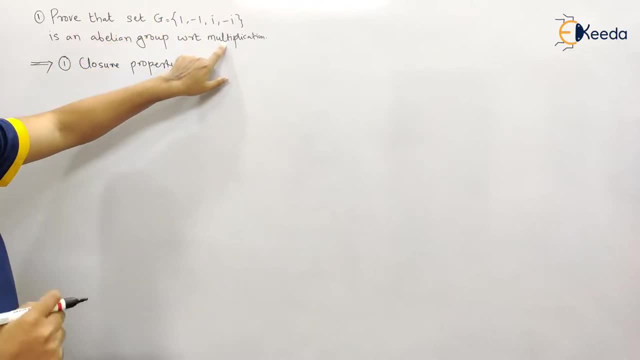 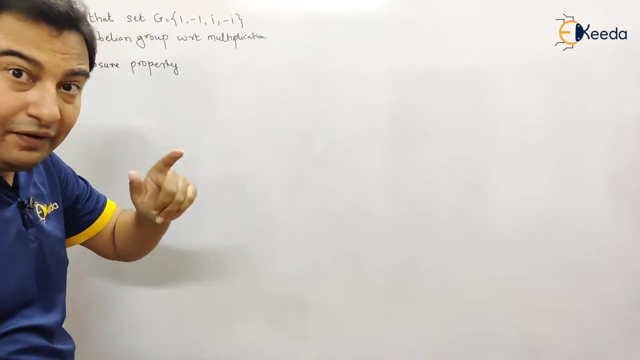 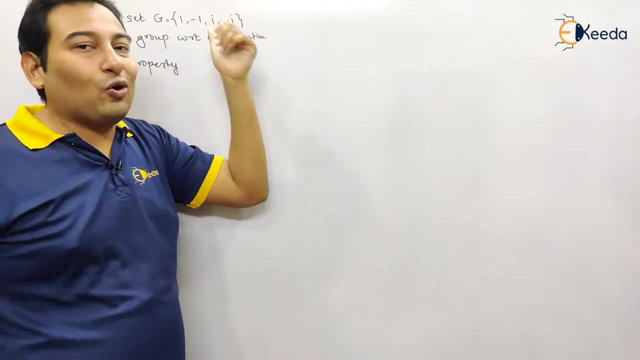 set and we applied multiplication operation, the result should also belongs to this particular set. I hope this is clear. Definition is clear. What is the definition? If we take any two elements from the set and we apply multiplication, the result will also belongs to the set. okay, so for that purpose, 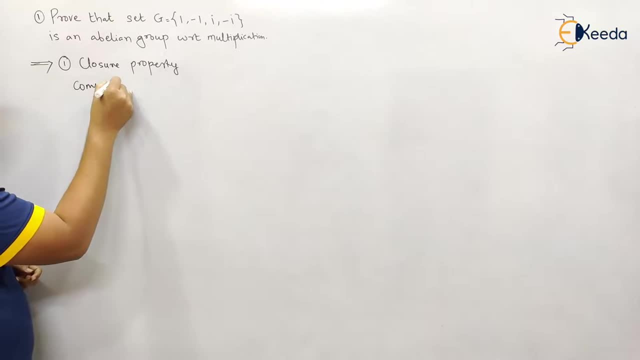 we going to form a composition table, because we need to check all the combinations. so let us form a composition table. so table once you are ready with the table. it will make your answer simple. so let us do it. the operation is multiplication. here the elements are 1. 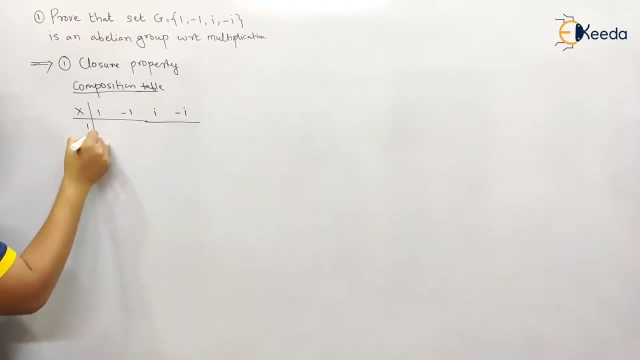 minus 1 i and minus i. 1 minus 1 i and minus i. let us multiply. so 1 into 1 is 1. 1 into minus, simply multiplication. one will be multiplied to all the terms. all the terms will remain, as it is minus 1 into all these terms. so minus 1, this will become plus 1, this will become. 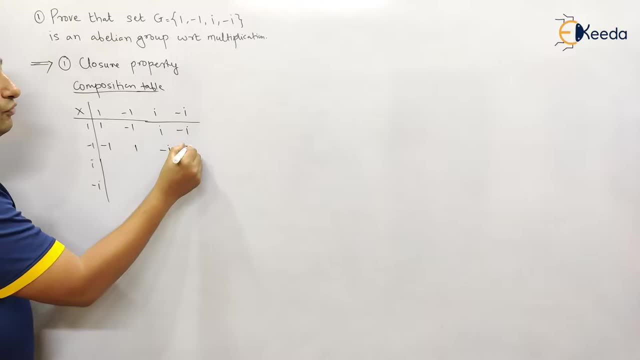 minus I. this minus minus will become plus and will be left with I. only next I. this is minus I. this is I square and I hope you know I square will be going to be minus I and plus value is minus 1. so this is minus 1 and this is minus into i square. i square value is minus 1. 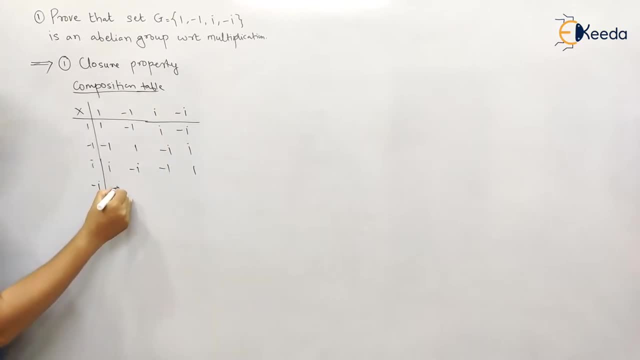 and also minus, so that will become plus 1. next minus i, minus, minus, plus i. this is 1, because minus i square, so that is 1 minus minus plus and i square value is minus 1. so this is your composition table. now check all the entries in this composition table belongs to this particular. 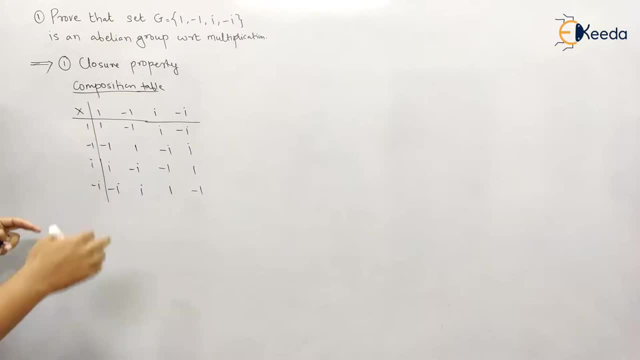 set. therefore you can say it is a closed. obviously that means you can take any two elements and multiply and result will also belong to the set, since all the entries in the table belong to set g. therefore g comma into is closed or basically it satisfies closure. property one and the same thing you can write on any other. 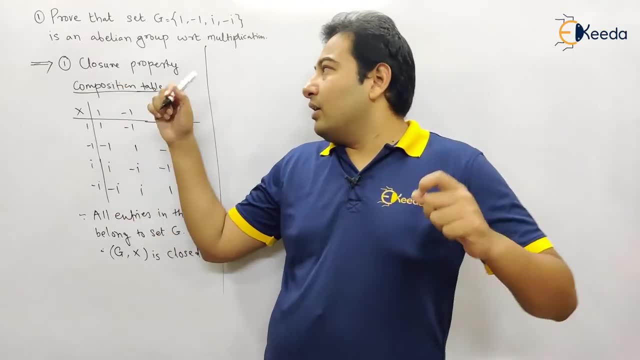 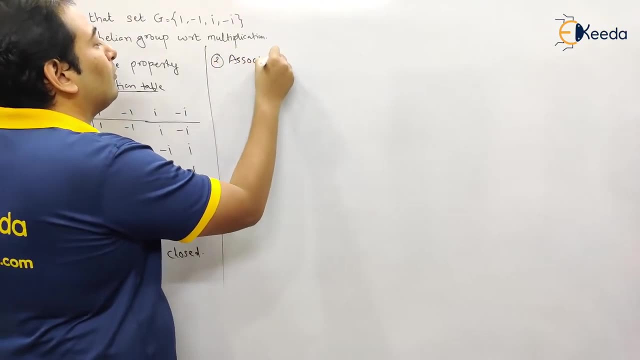 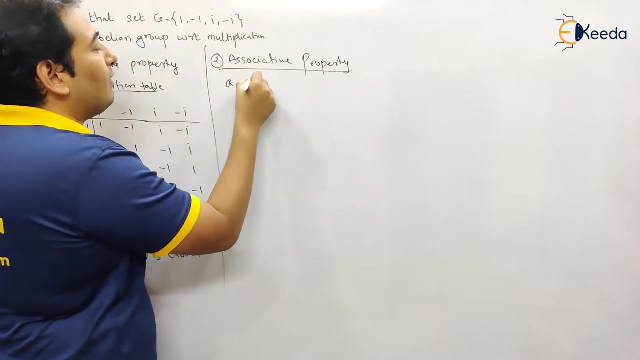 anyway. okay, let's move on. so we discussed the closure property. what is the next property? associative property. so what is the associative property? associative property is very simple and the property says a star b, star c. you can write it down as a star b, star c. so for proving, 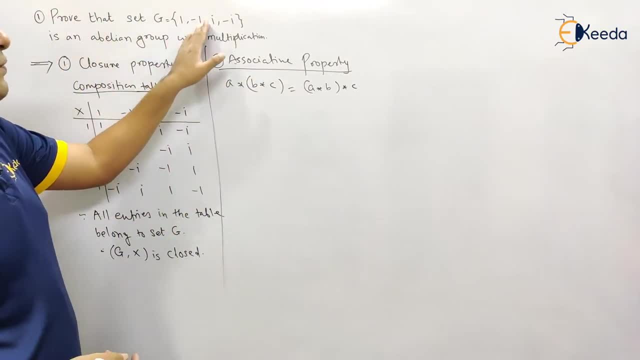 associative property. you can consider any three elements from this set and check whether it is satisfied or not. so this is one option, so let us do it. consider any three elements. so let's take 1 minus 1 and i you can take any three elements. so let me take 1 and star is obviously into now. 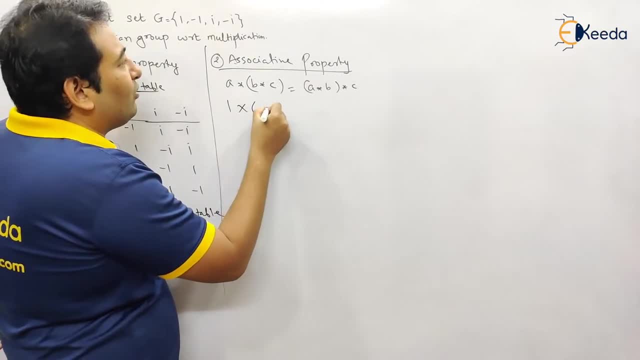 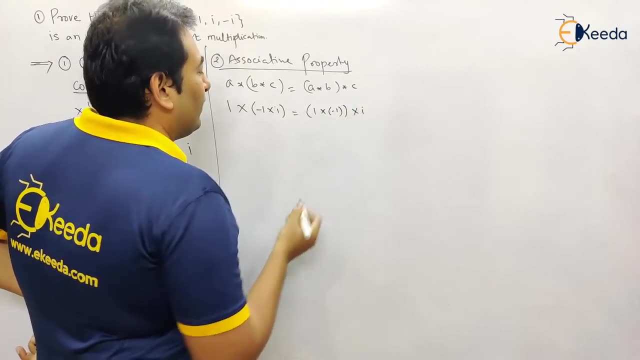 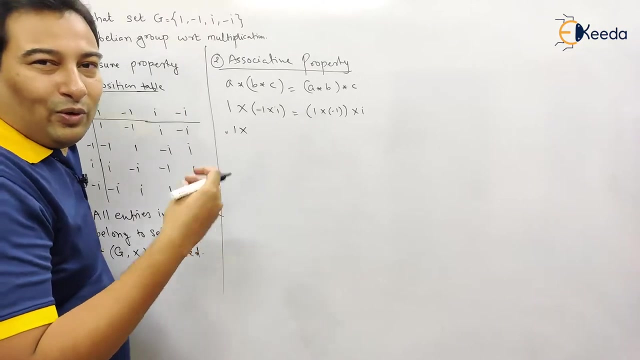 multiplication, because it is given in the problem, and minus 1 into, let's say i. 1 into minus 1. so minus 1. we need to write it down in a bracket into i. so here first of all the bracket will be evaluated. so minus 1 into i, minus 1 into i. you can do it orally. that is minus i. but ideally 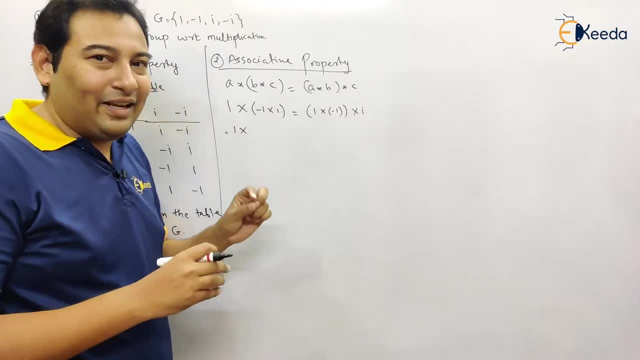 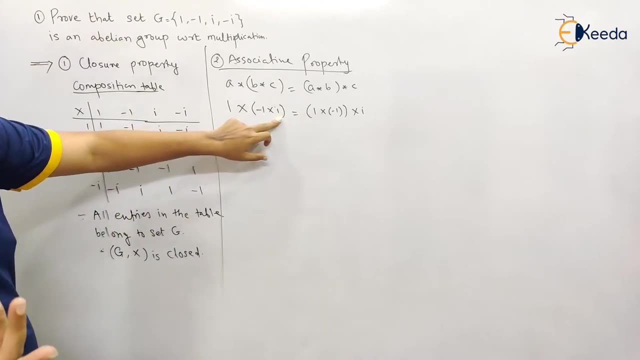 this is very simple. you can easily manage by yourself. but ideally when the problems are complicated, we refer the table for that purpose. we have already table. so minus 1 into i is obviously minus i. but let us check in the table: minus 1 into i is minus i. so this is the way we're going to do. 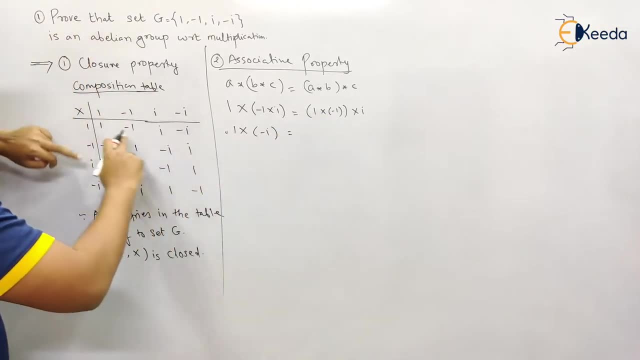 it. 1 into minus 1. obviously minus 1, but still check: 1 into minus 1 is minus 1, because when the problems are complicated you should know how to use the table. so 1 into minus i. so this is 1 minus i. this. 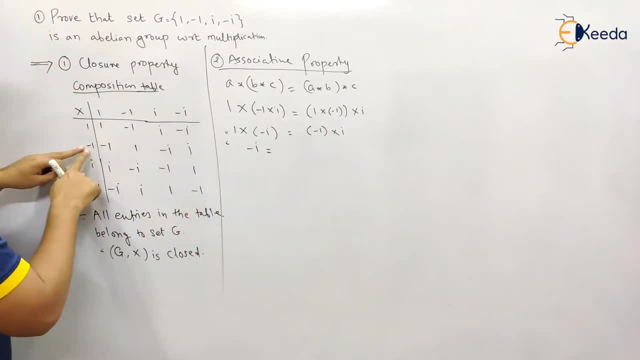 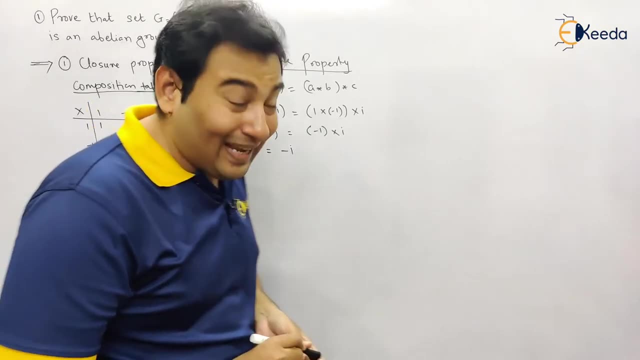 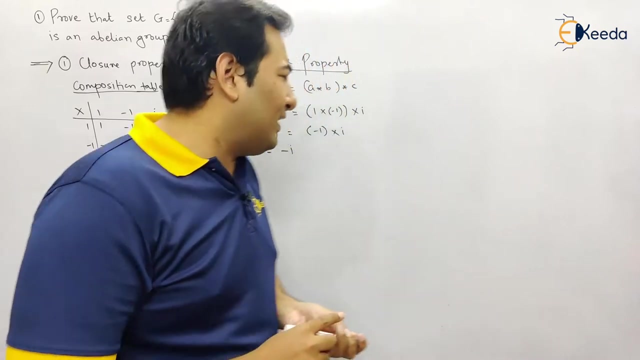 is minus i equal to minus 1 into i. so minus 1, i is again minus i. so see here, therefore, associative property satisfied. so you can take any three elements from the set and you can prove associative property. or simply you can write it down as, since it is multiplication: 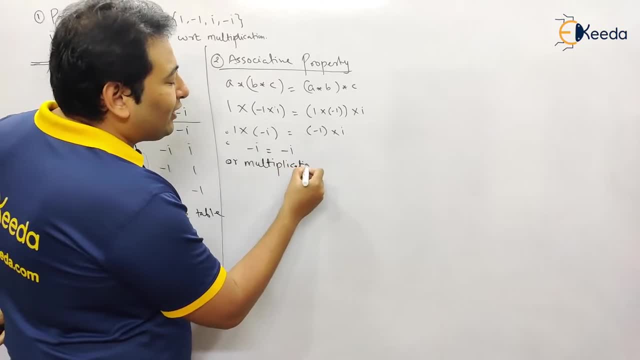 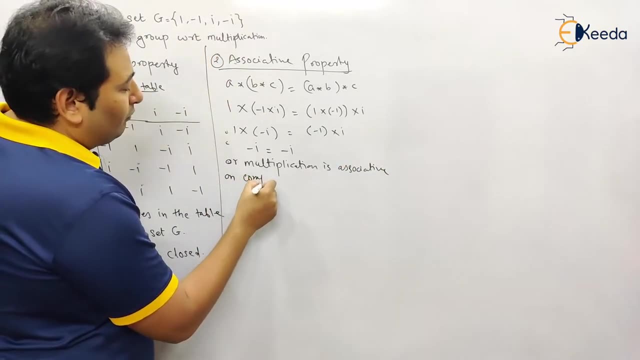 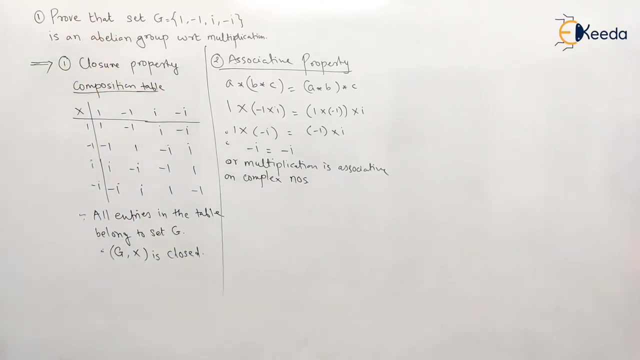 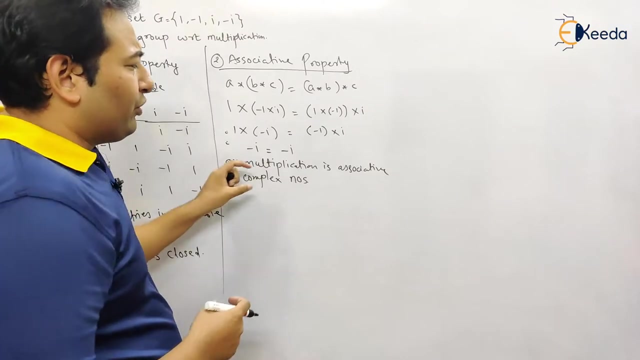 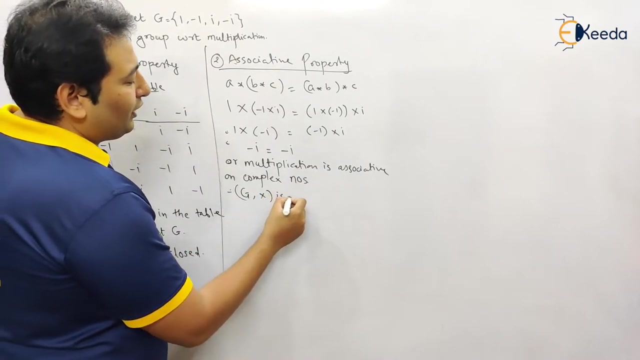 so you can write it on this point also. multiplication is associative on complex numbers. multiplication is associative on complex numbers with this point, or by pasta, by by. by this you can say therefore, G, comma into is associative. what is the next property? if it is asked to prove semigroup, we are done with the solution because semigroup 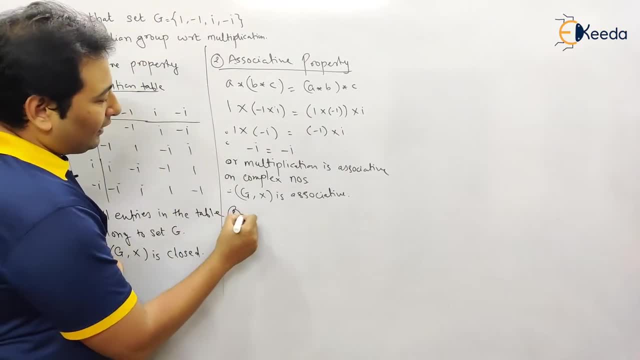 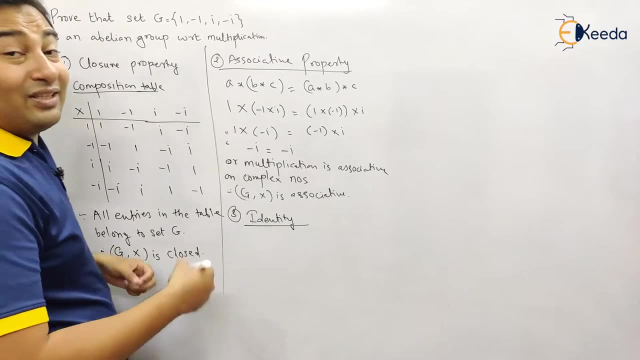 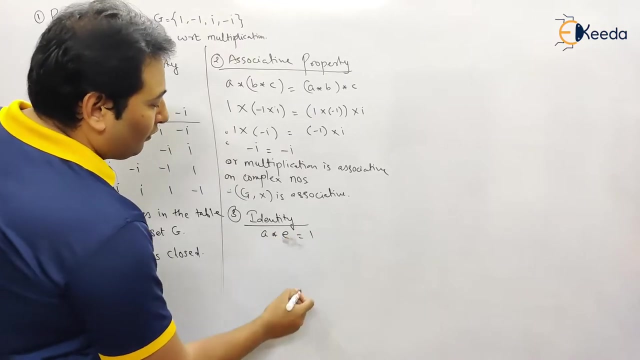 means only satisfying two properties. the next is identity element. if you prove that there exists an identity element, then we can conclude: yes, it's a monoid. so let us start. what is the definition? a star e is equal to a. a star e is equal to a, so a means the element. so here there are four elements, one minus. 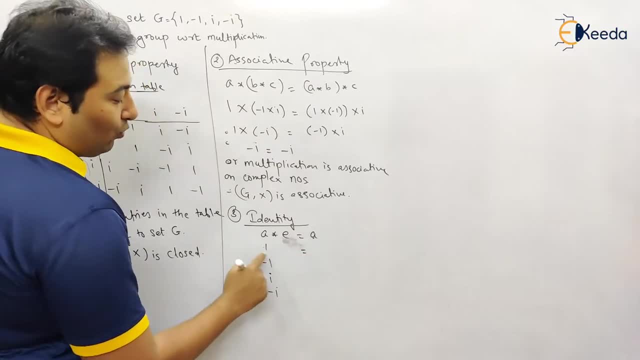 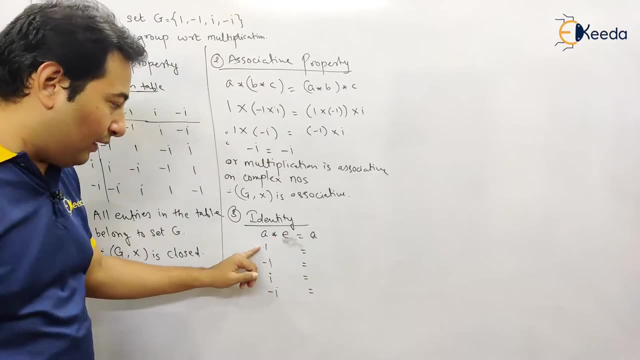 one I and minus I, equal to on right hand side. you should get the same term. see here: if we have a on right hand side, you should get the same term. so if it is one, you should get one minus one I and minus I on right hand side, you should get the. 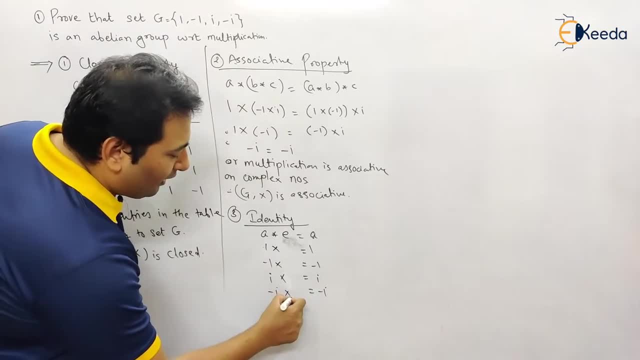 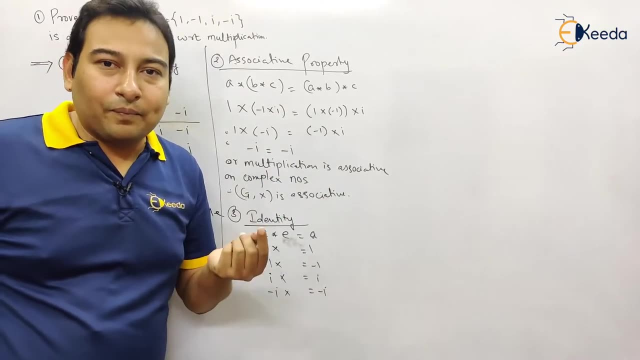 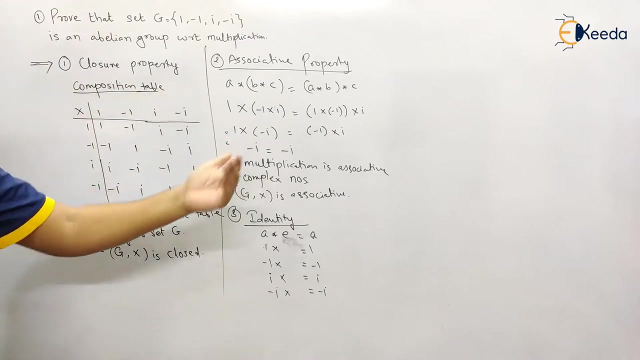 same term and operation is multiplication. now we know, as discussed in the last video, also with respect to multiplication, what is the identity element. it is one that we know, we can write it on one simply here, but still we will check with the help of a table so that when, whenever the complicated problems, 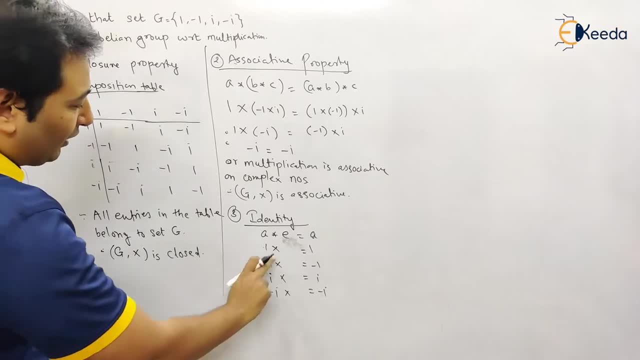 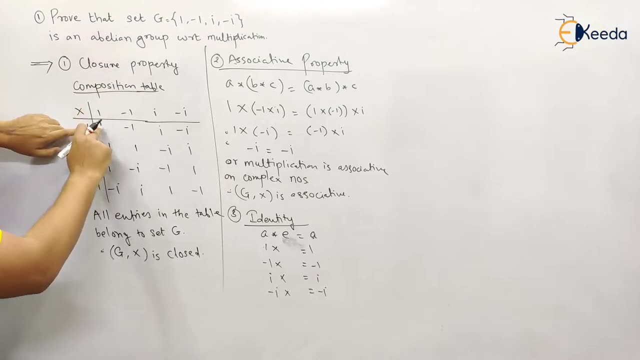 will come in the exam. we should be able to understand how to use this table. so, 1 into what is 1, see here 1 into what is 1. so 1 into 1 is 1. next, minus 1 into what is minus 1. so minus 1 into 1 is minus 1. so again here, minus 1, obviously 1 will. 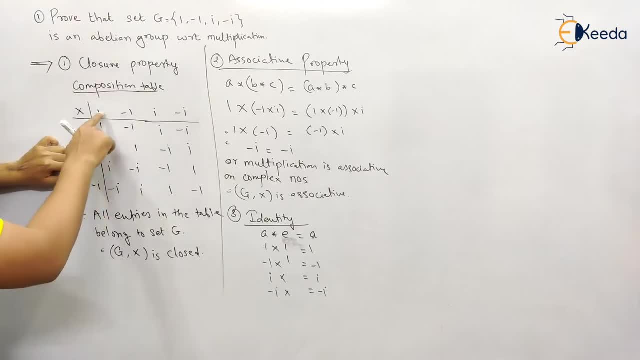 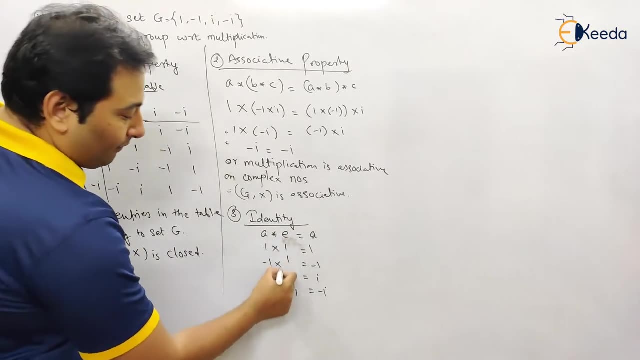 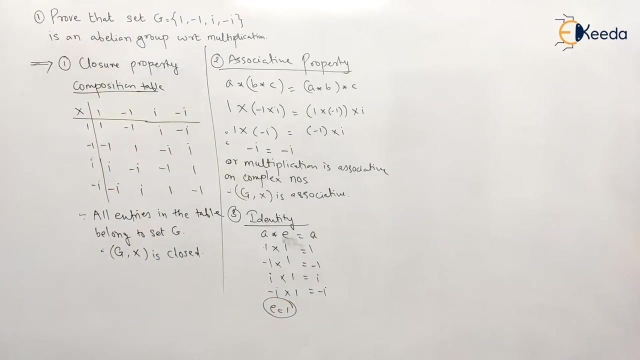 come everywhere, but still I into what is I? so I into one is I, and likewise, minus I into 1 is minus I. so that means: see here e is equal to 1. so we got the identity element, and the identity element is E, which is equal to 1. that 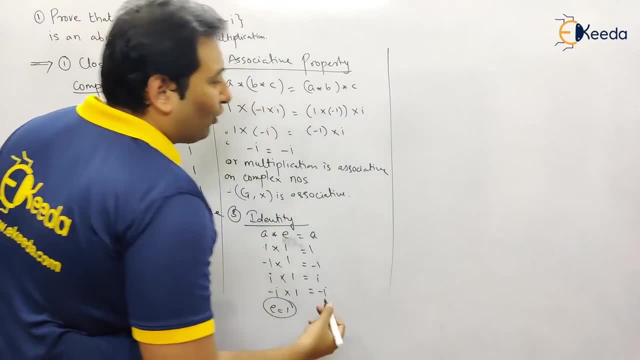 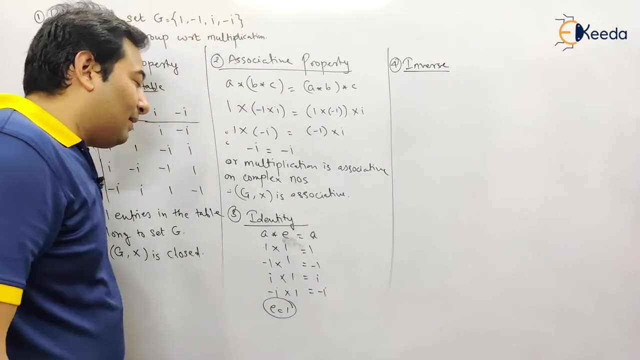 means your same. a group now became monoid. let us move on. let us discuss inverse. if inverse exists, then the monoid will became, will become group 2., 3, S, 3., 4. and so on. what you need to do is to divide 3.. 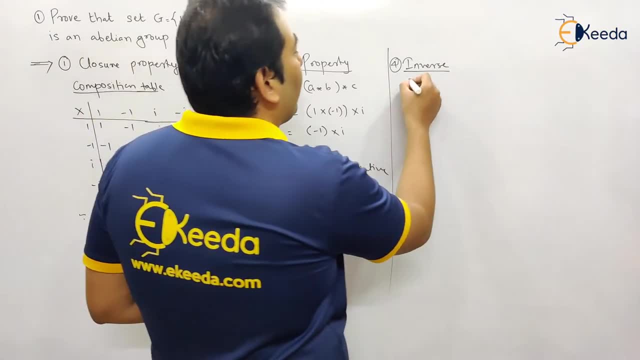 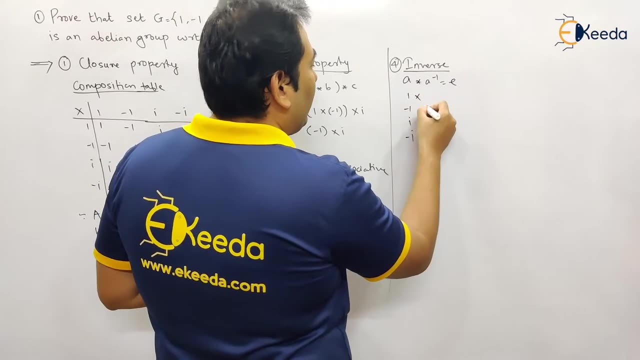 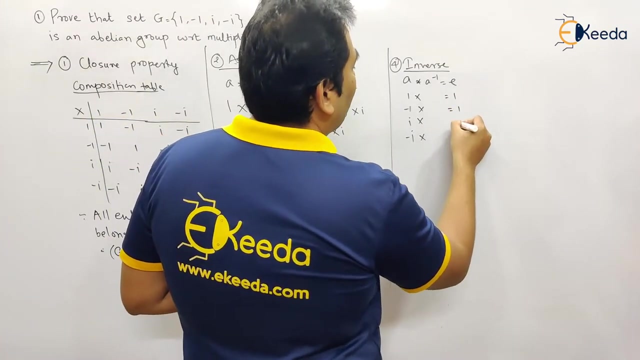 group. so what is the inverse? a star, a inverse equal to e. so there are four elements: one minus one i, and minus i into is equal to e. e should is your identity element and we found out e is one. so on right hand side we should get one. so let us find it out. inverse of each and every time. 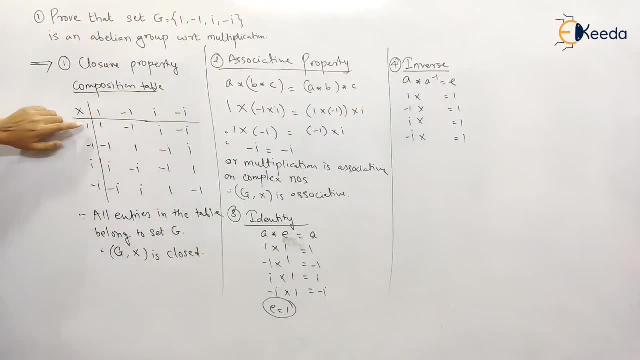 so how to check one into what is one? see here one into one is one. so here one will come. next, minus 1, into what is 1 minus 1, and see: here it is 1. so minus 1. into minus 1 is 1. so here it will be. 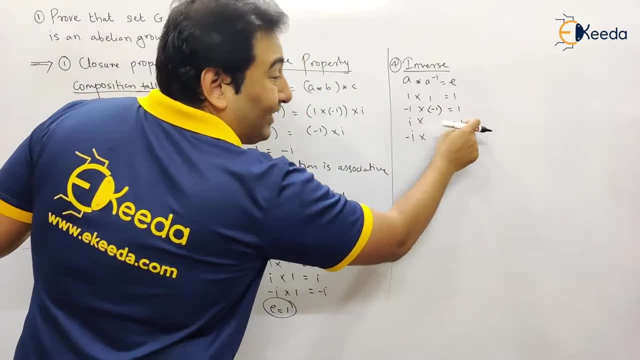 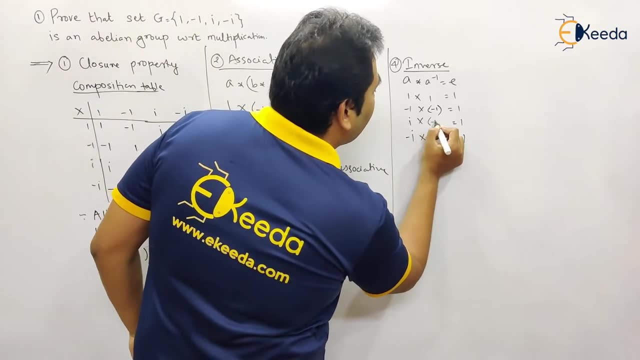 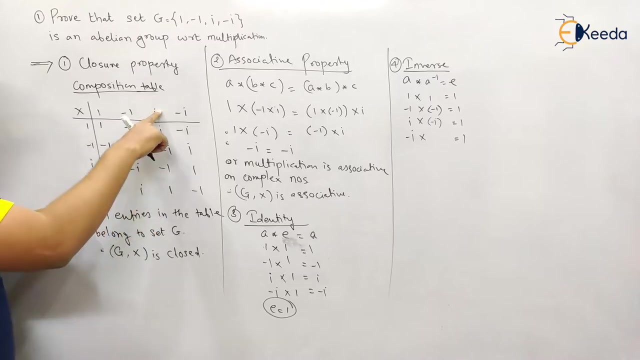 minus 1. next i into what is 1. see here: i, this is 1. so i into minus i is 1. so therefore minus, i will come here. and finally, minus i into what is equal to 1. so minus i in 2, i is equal to 1. that means 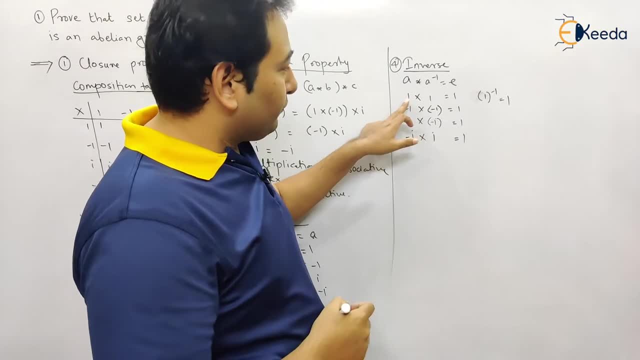 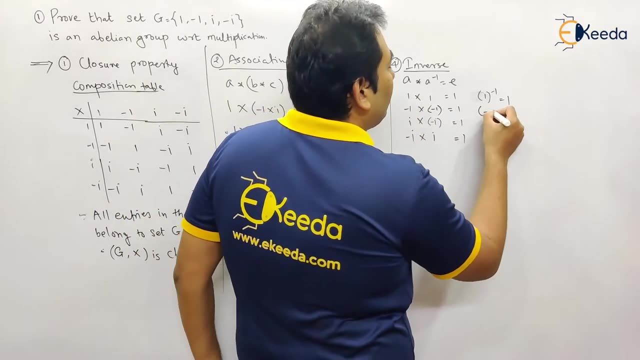 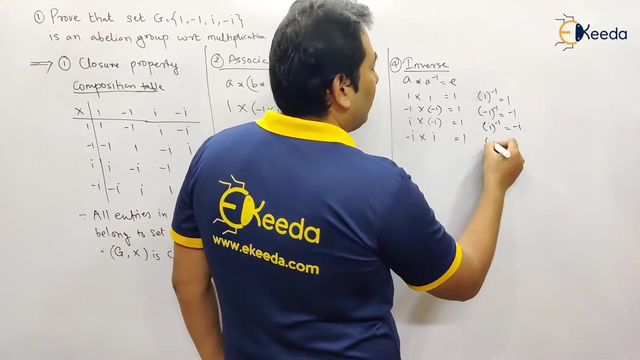 1 inverse is 1. see here, this is the term, this is its inverse, so a and a inverse. so 1 inverse is 1 minus 1. inverse is minus 1. i inverse is minus i and if you check here, minus i inverse is i. that. 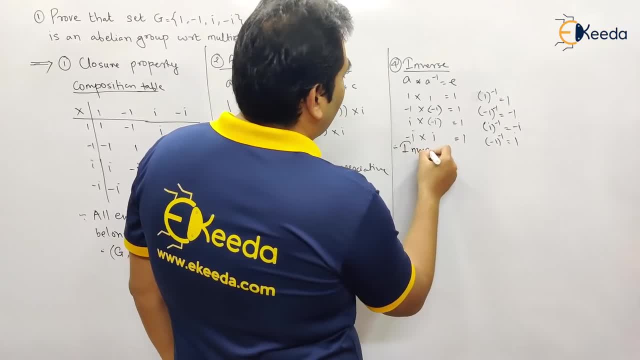 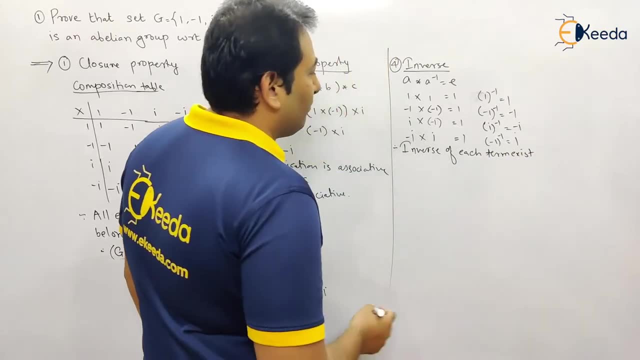 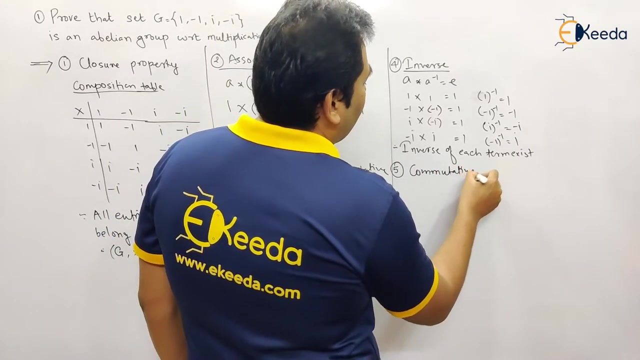 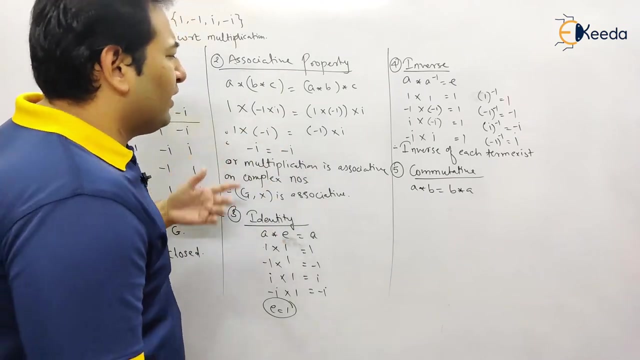 means inverse of each term exists. that means your monoid becomes: become group, became group. now let us discuss last property that is committed to. if it is also satisfied, then you can say it's an abelian group. a star b is equal to b star a. very simple property. you can take any two terms and you can prove this. let me take 1 and